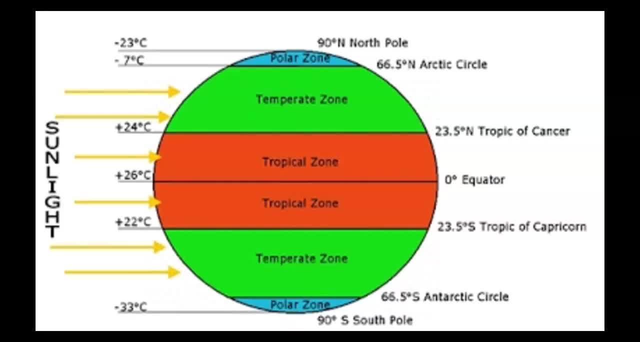 Antarctic Circle. There are 3 climate zones. One Tropical Zone zone is also called the torrid zone. Two, temperate zone. Three, polar zone. The polar zone is also called the frigid zone. Tropic zone: The region between the Tropic of Cancer. 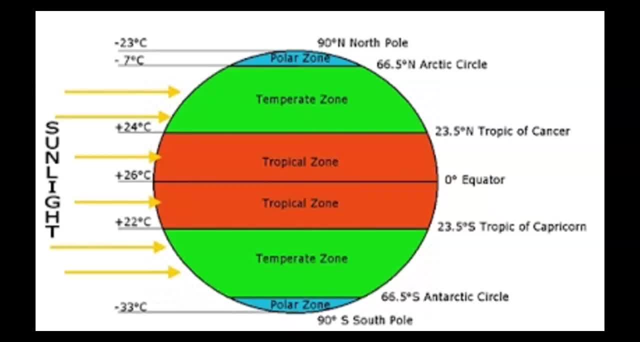 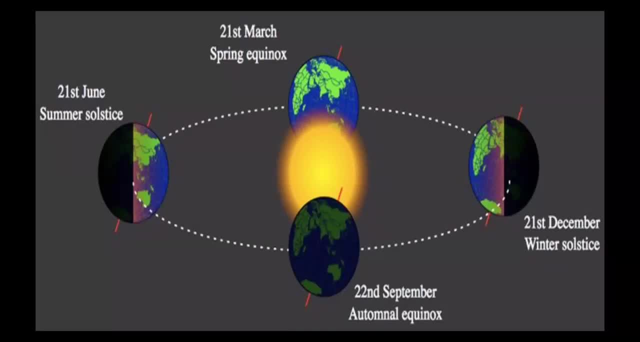 and the Tropic of Capricorn is called the tropic zone. This is the utterest part of the earth. The sun's heat falls directly on this zone during the solstice and the equinoxes. The summer solstice is the time of the year when the sun passes overhead the farthest. north. It usually takes place on the 22nd of June, And the winter solstice is when the sun passes farthest north. The summer solstice is the time of the year when the sun passes overhead the farthest south of the equator, which usually happens on the 21st of December. 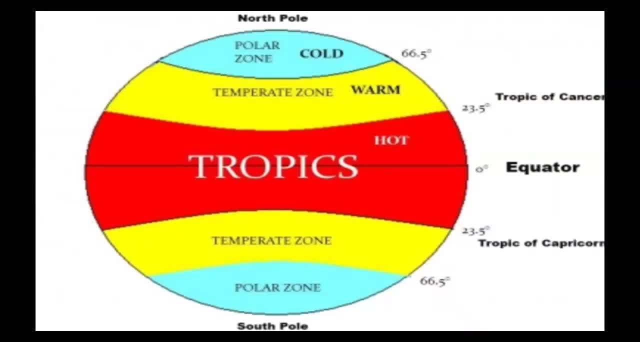 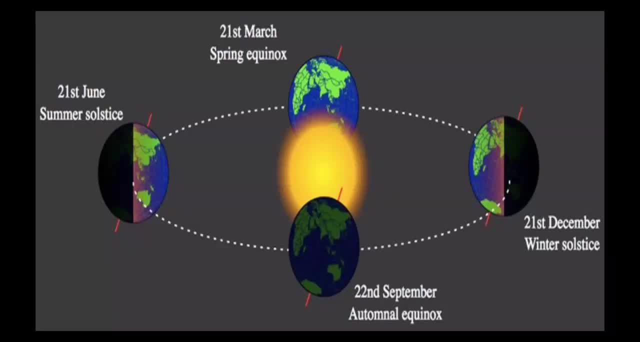 The equinoxes usually occurs two times each year. This occurs when the sun crosses the equator and day and night is approximately of equal length. almost The cloven solstice is when the sun crosses the equator and day and night is approximately of equal length, and the 50th is when the sun passes overhead the farthest south of the equator, which is 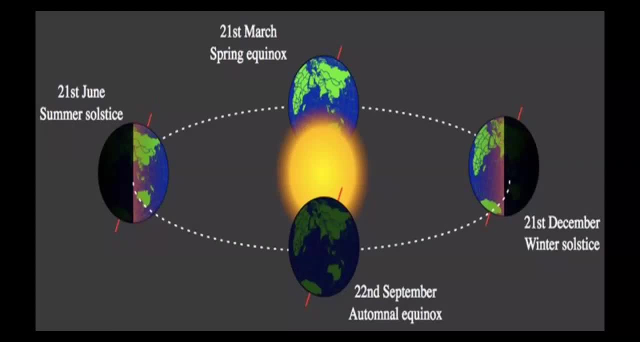 considered to be on the earth. However, one day of the year the solstice is not known today, because the selner solstice occurs every 10 days and there are also times when there is no solstice: forext sóaur. This usually happens on the 21st of March and the 22nd of September. This usually happens on the 21st of March and the 22nd of September. The tropical zone includes Jamaica, the Caribbean, most of Africa, southern India, south Asia, Indonesia, Victoria and заявes that Raise, the book of Ofamily, has a pretty important version of the tropical horizon. 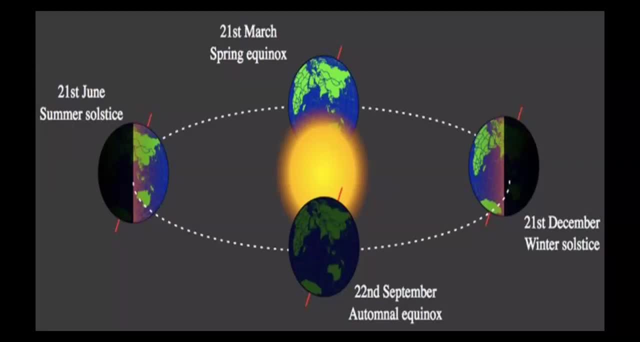 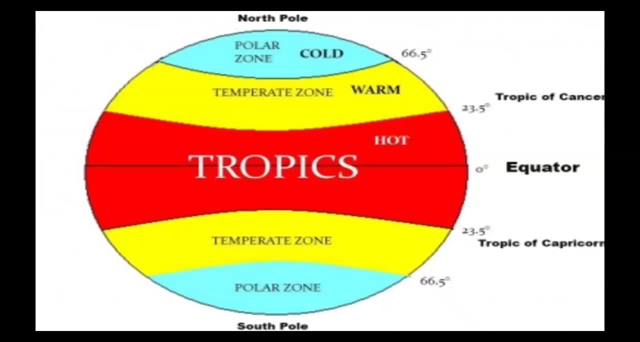 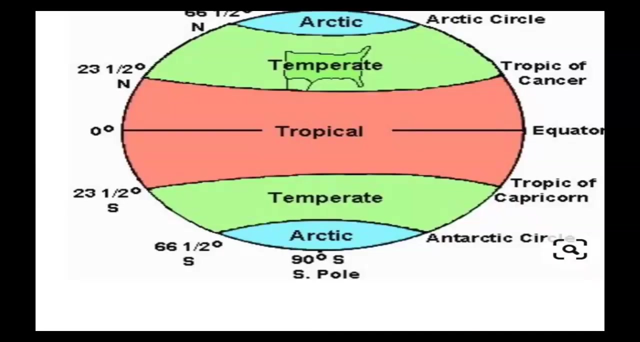 For that reason the tropical zone is not intended to be adjudicated places or where остановca in South Asia, Indonesia, New Guinea, North Australia, Southern Mexico, Central America and Northern South America. The second zone is the temperate zone. The temperate zone falls between the two tropics and the Arctic Circle in the north and the Antarctic Circle in the south respectively. This zone usually has a mild temperature and enjoys all the four seasons annually: summer, spring, autumn and winter.